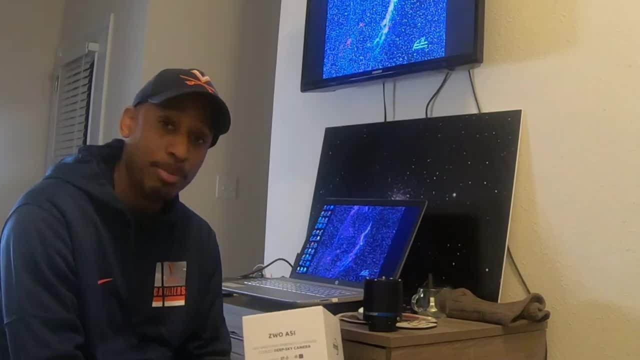 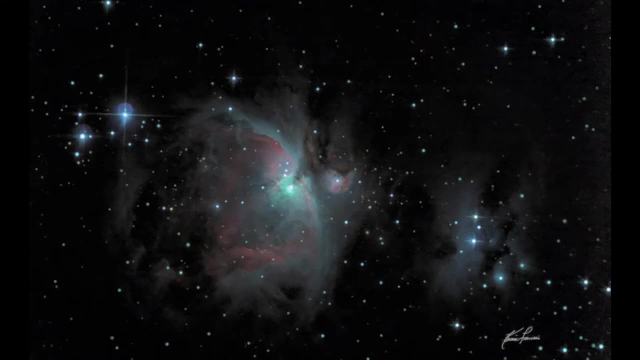 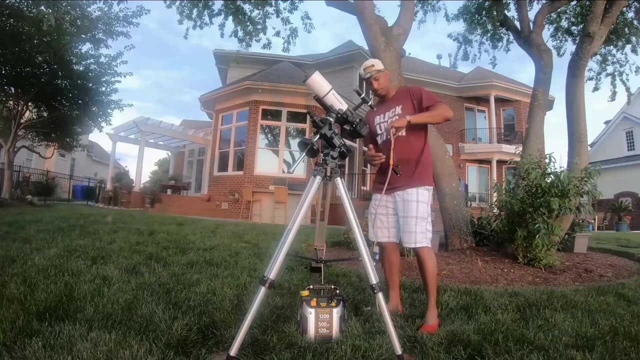 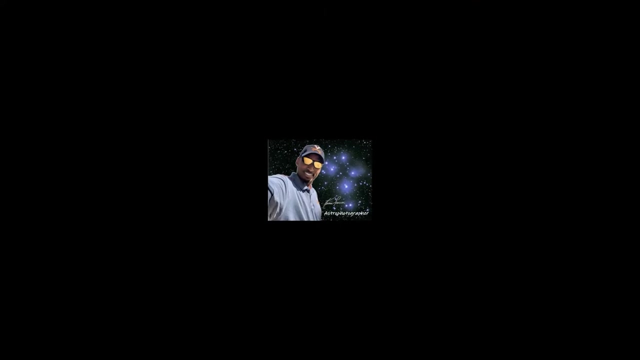 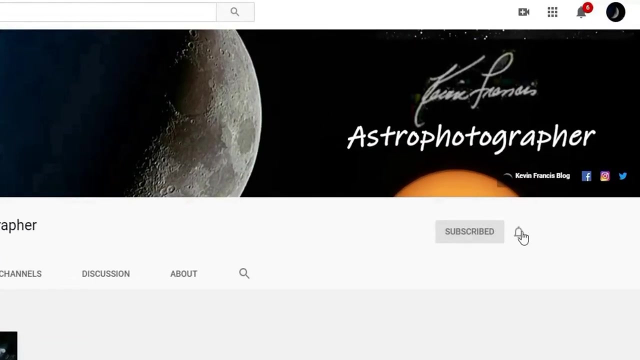 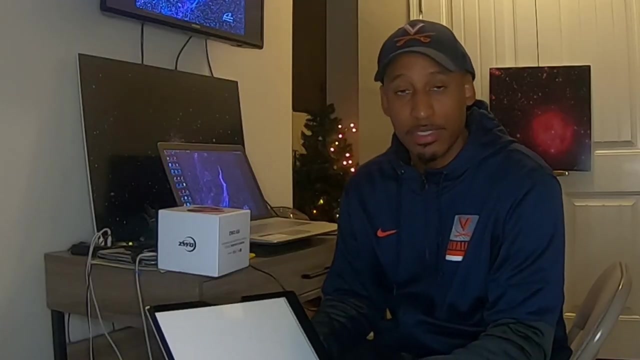 We're going to talk about how to calculate any of the settings that you would like based on using Excel. Get ready. This is going to be pretty technical, but I think you'll like it. So, to get ready for your sensor analysis, you're going to need a few things. 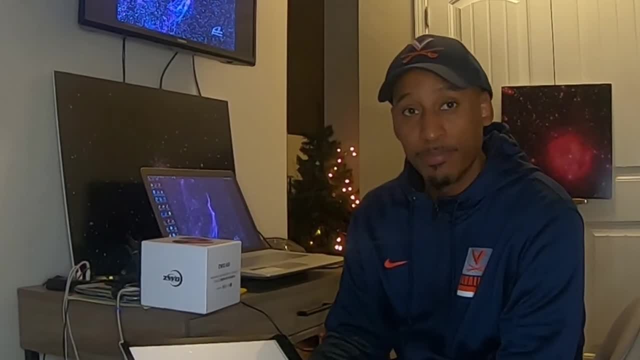 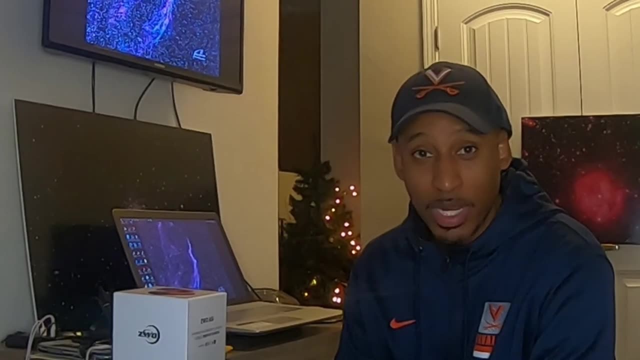 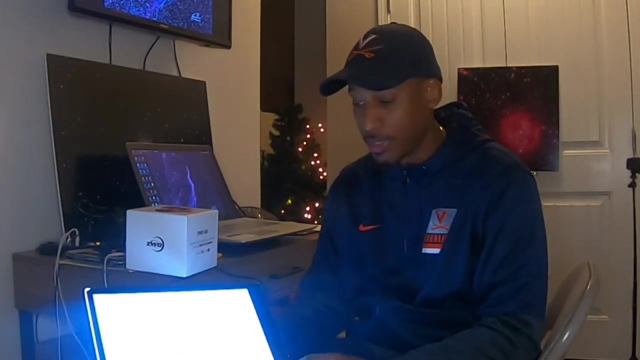 One. you need a light source. You could use an iPad, for example. I bought this sketch board from Amazon for less than $20. So I can turn this on and I can vary the brightness by holding this button. So I want this to be as dim as possible. 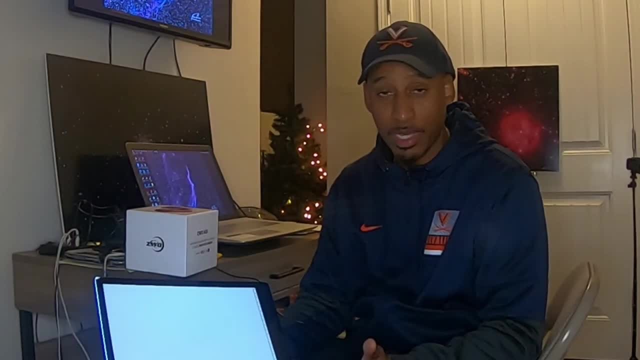 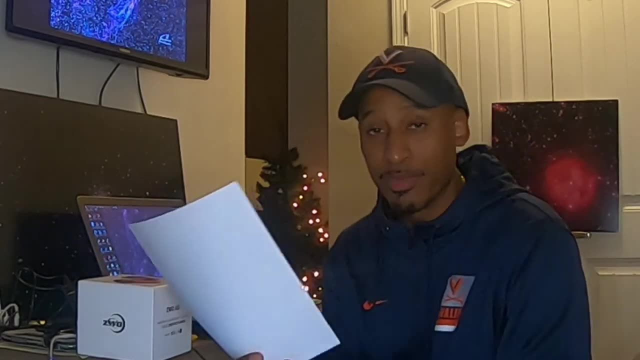 I also use this for my flats when I'm doing my hospitality sessions, but this is my light source, So you're going to need that. And then you're going to need a handful of blank sheets of paper- Doesn't matter the size, just as long as it covers your sensor, because 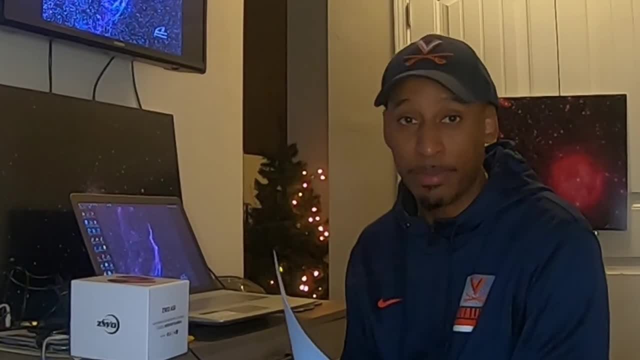 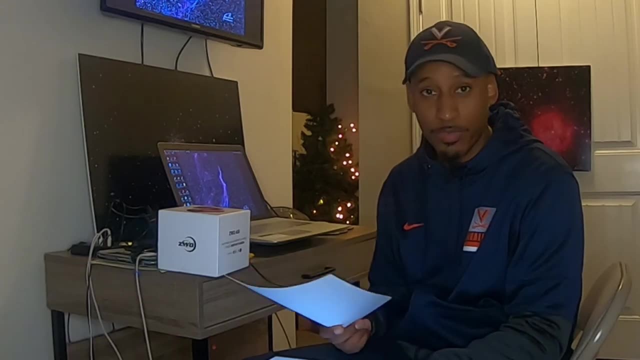 you've got to get to a low enough light level for a sharp cap to do this work for the sensor analysis, So make sure you have those. Some people use a white sheet that you can fold a few times so you get to that right brightness level. 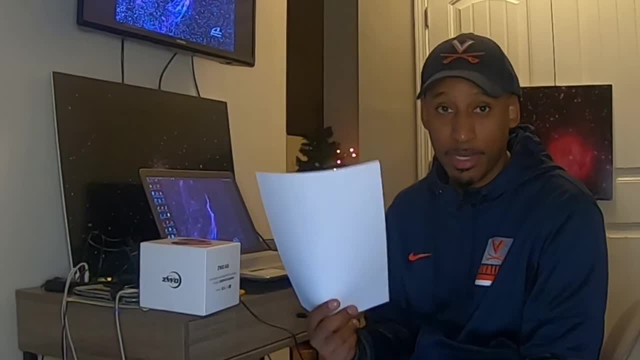 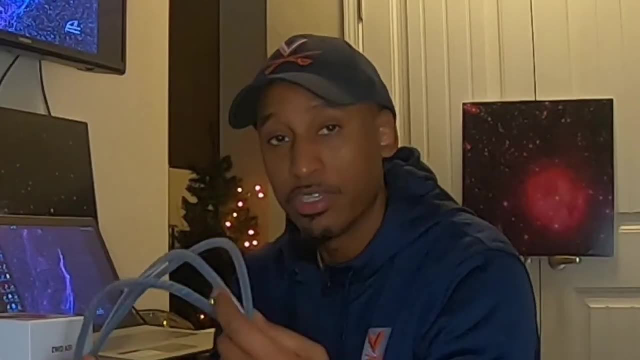 But I use paper. It works great As long as it's blank. you're going to get an even view of the light all across the sensor for the analysis. You're also going to need power and USB for the camera. You can connect it to your laptop. 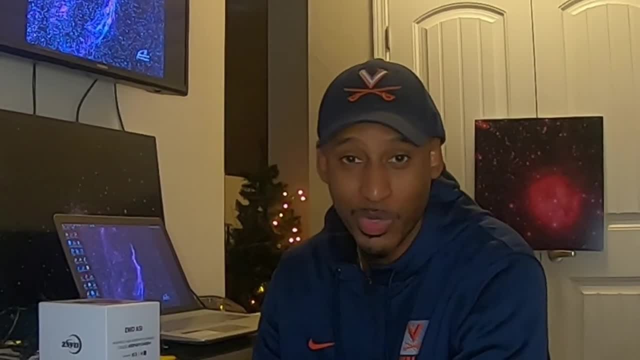 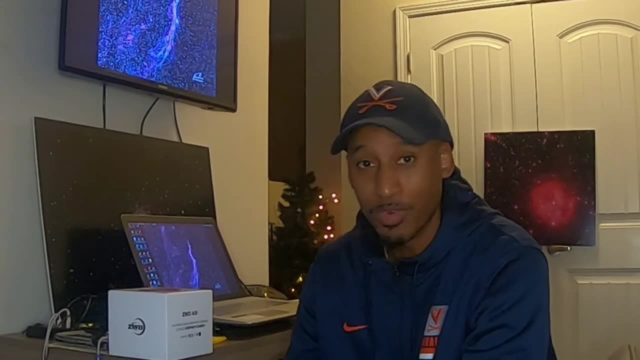 and you can cool it down, especially if you're inside. You still want to cool it down to about zero at least to do this session. It has no real advantages, but to keep your camera from overheating for no reason, it's a good idea to just go ahead and let it cool. 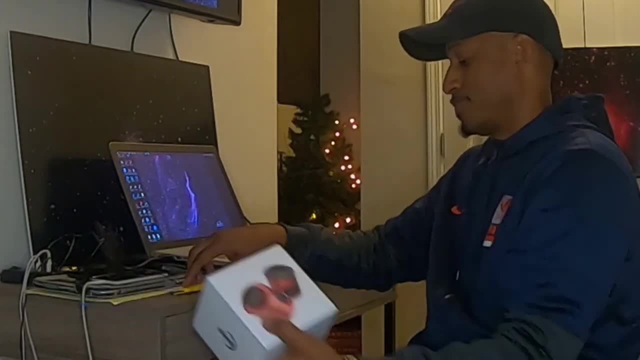 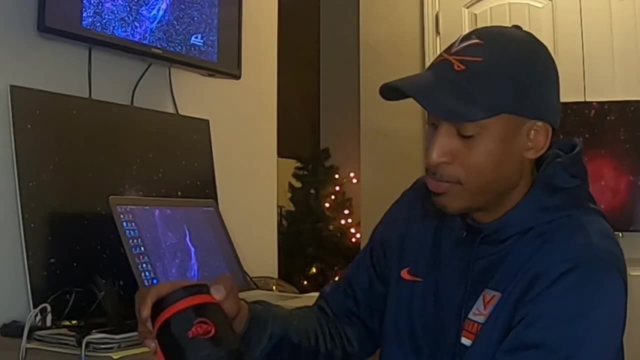 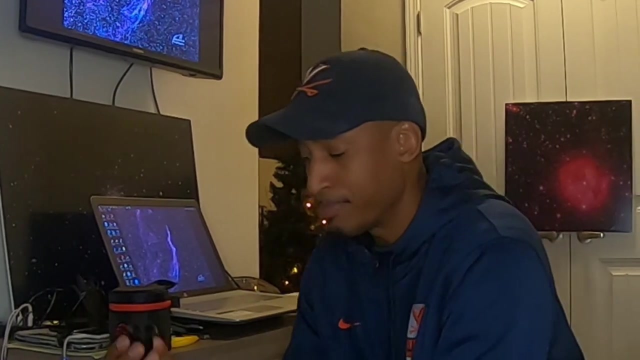 So great, Let's open this up. Ah, that new camera smell. So if you've not seen a ZWO camera before it comes in a lovely little case, We'll pull that out, And it's got a bunch of different accessories in here. 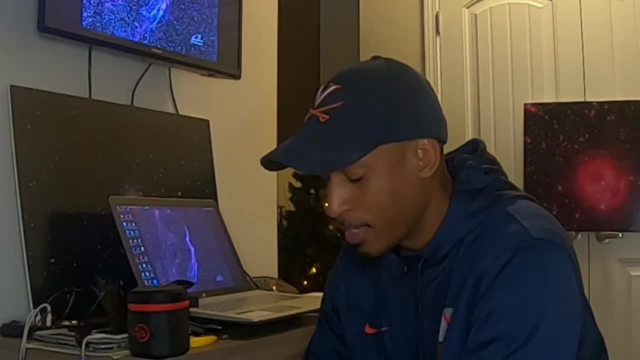 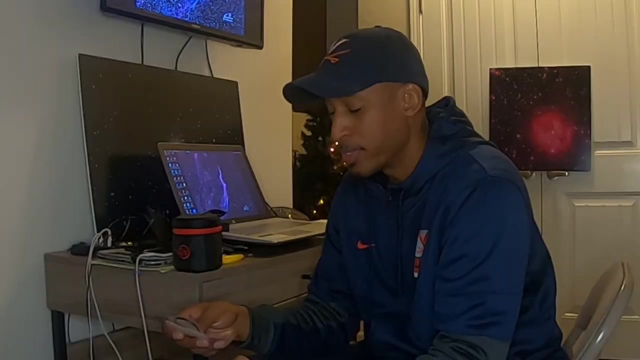 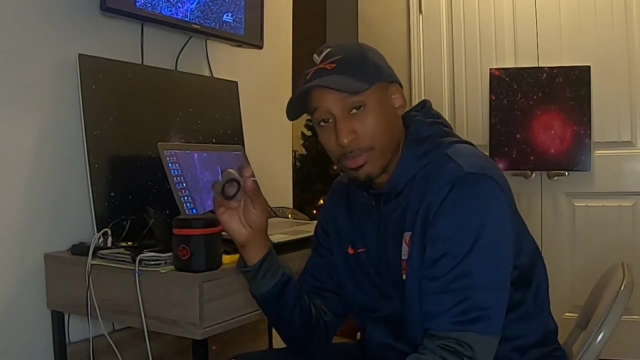 adapters that you can use for your different setups. spacers as well, if you need them for back focus. USB 2 and USB 3 cables for the camera. ZWO- here There's a few more spacers for getting your back spacing correct, And this is actually a nice little gift: It's a 1.25-inch filter. 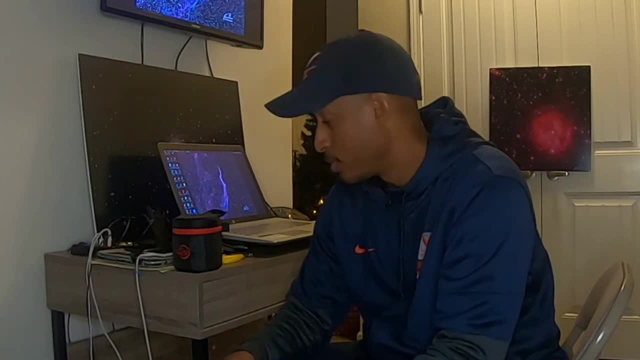 holder. So that's a good addition. You don't have to buy a 2-inch filter for that size camera sensor. And of course, it comes with a quick guide. All right, quick unboxing. So now that you got your camera out of the bag and out of 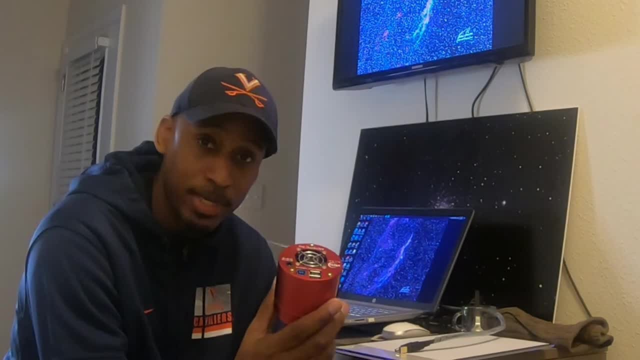 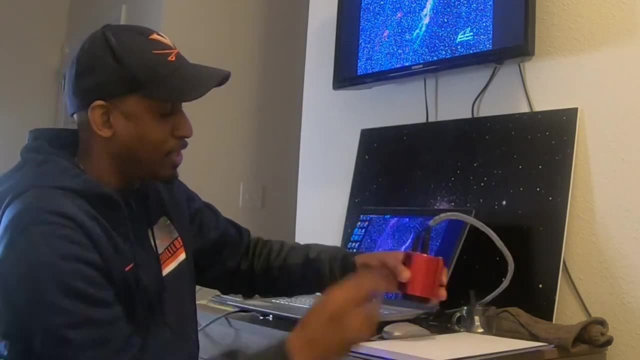 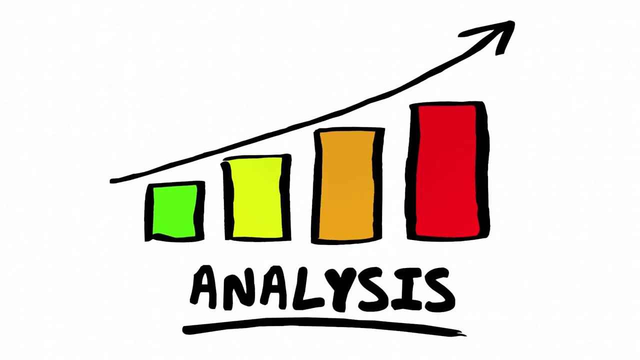 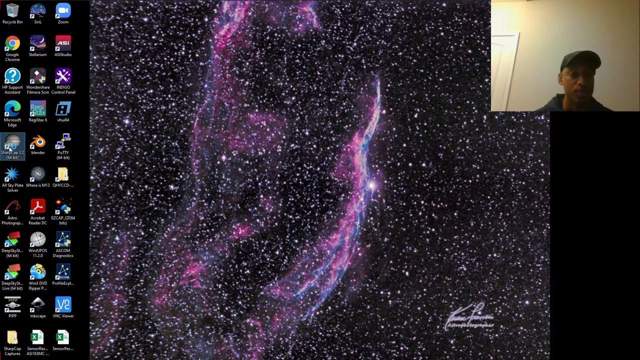 the box. really simple setup: You're just going to plug it in, You're going to leave the cap on and then we're going to follow the directions on SharpCap. That's it. I'm going to open up SharpCap. I've got everything connected. I've got my light source turned. 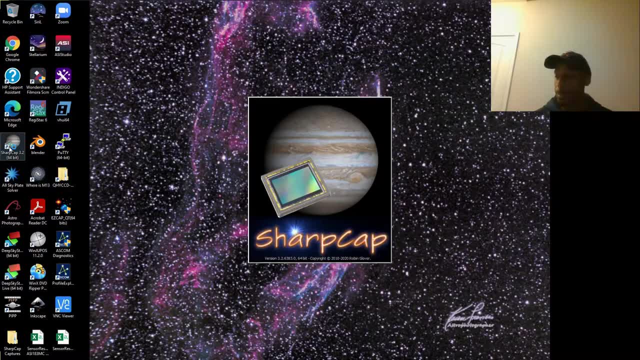 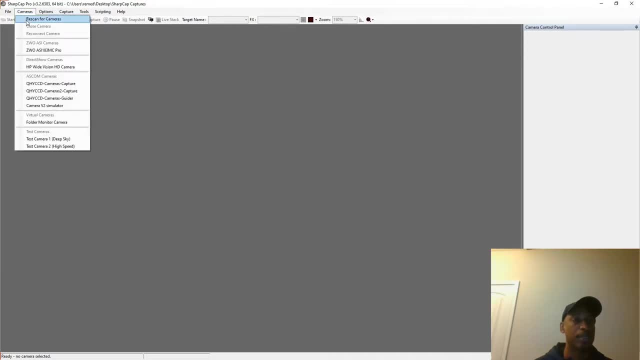 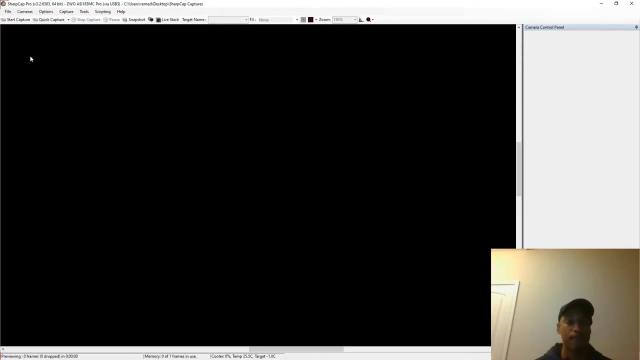 on. I've still got my camera capped right now, So that's okay. Okay, so now we've got SharpCap open, Let's go ahead and connect the camera And see it's here, the ZWO ASI 183 MC Pro. Click on that. All right, now it's connected, So we're going to go to Tools. 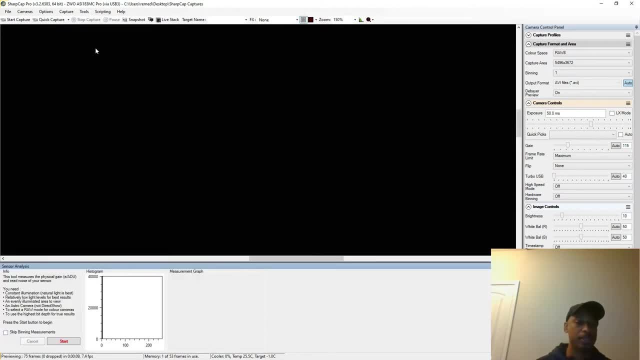 and Sensor Analysis, And this begins at the bottom by giving you a measurement graph, And this is the measurement graph with the histogram, And it tells you that you need constant illumination- natural light is best. So, since we don't have natural light and 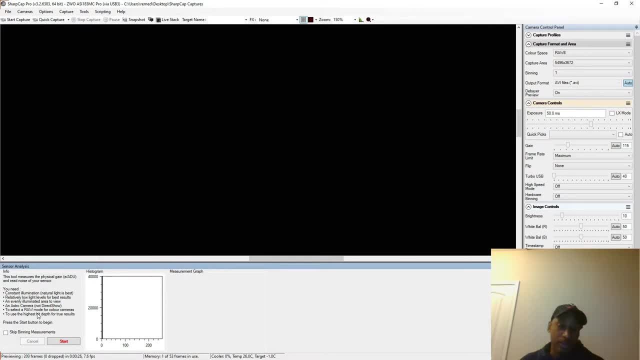 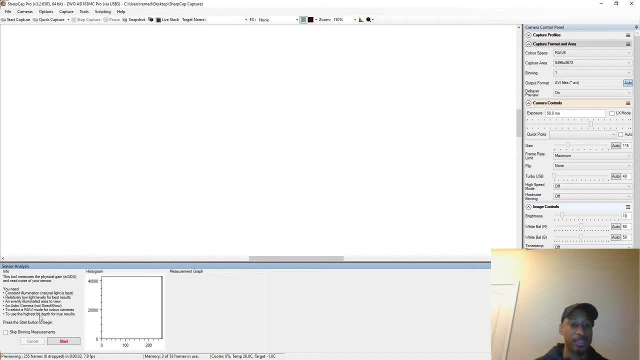 we're using this pad. we're going to start there. First things first. we want to take the cap off. All right, now that's telling you you've got way too much light because that bar of histogram was here to the left, Now it's over here to the right. Okay, let's. 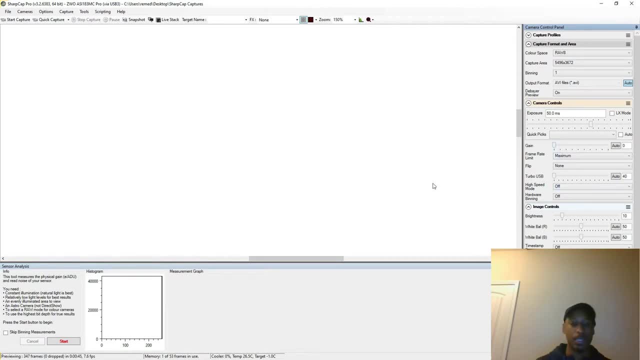 turn my game on Down zero. Now I have this as low as I can get it, I'm raising it up. This that I'm talking about is my light source, So that, as low as I can get it, I need to change my color space. 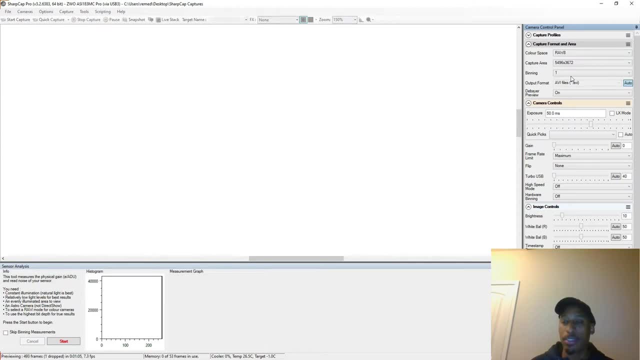 to raw 16.. That's what the camera uses, Okay, And so I've got these capture areas, So I'm going to go ahead and hit start So you can see what I've set here. Okay, now we're going to go ahead and set this image to the highest one possible, Very large capture areas. So 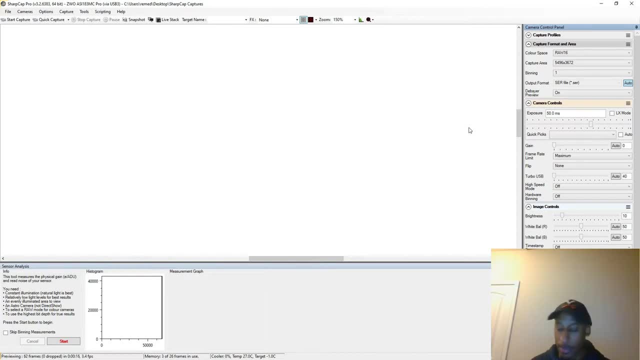 right now it's set to the highest one possible. Okay, All right, So good, Let's go ahead and take this, because we want this histogram to come down to about 60% And this will tell us that. so let's hit start So it can tell us that. All right, so we're going to select. 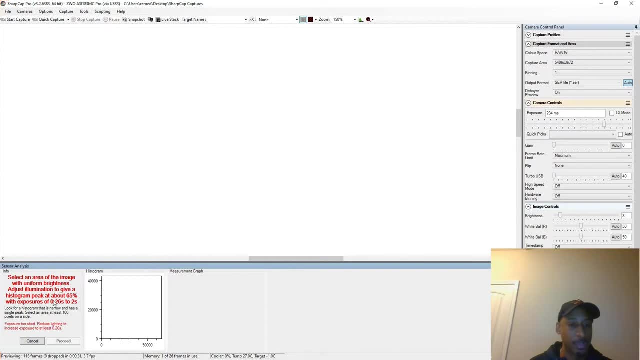 an area of the image with uniform brightness. adjust the illumination to get a peak of about 65%, With exposures anywhere between 0.26 and 0.4.. So you can see that the image is in an area that's just right. So I'm going to click OK And then this will tell us what the image. 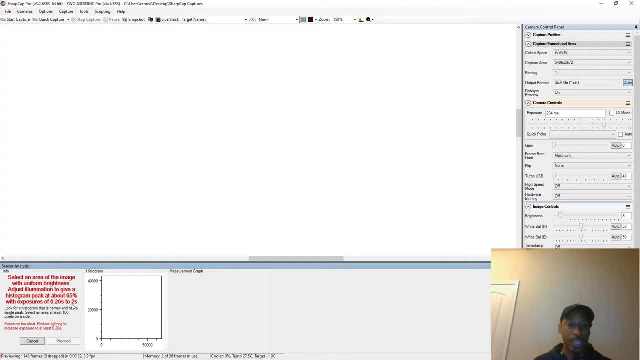 2.26 seconds and 2 seconds. We have a nice large range there, And so right now it's running. it's at .23 seconds or 234 milliseconds, So let's get that histogram down. So I have two sheets of paper. I'm going to put it right underneath: Start: Okay, so far, that made. 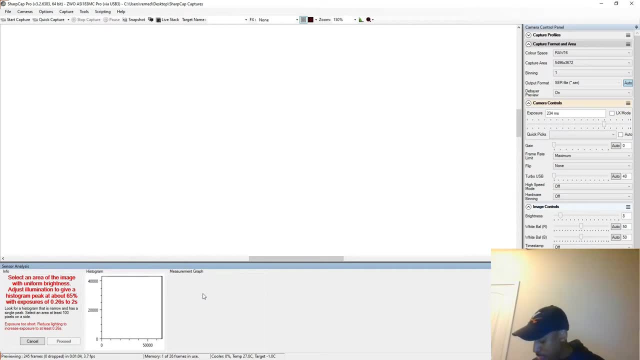 no change, Let's go a little bit higher. Two more, Okay. so now it's down, came down. The exposure time is still 234.. So we need to get that a little bit higher. So let's try. one more sheet of paper. 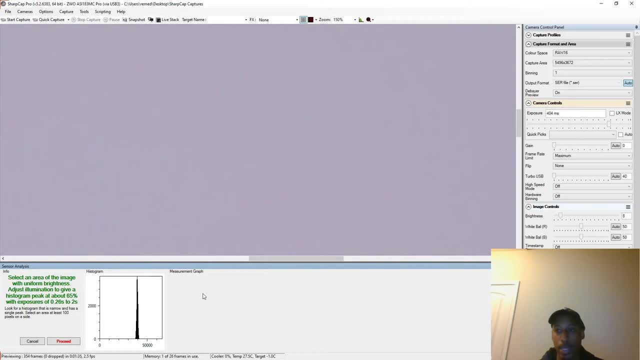 We're sitting at five sheets of paper. Now we're at .4 seconds. It's gone green. If you look down here in the bottom left corner now it's green. Okay, that means we can proceed. So we're going to click proceed And then this is going to go through. this analysis it's going to start. 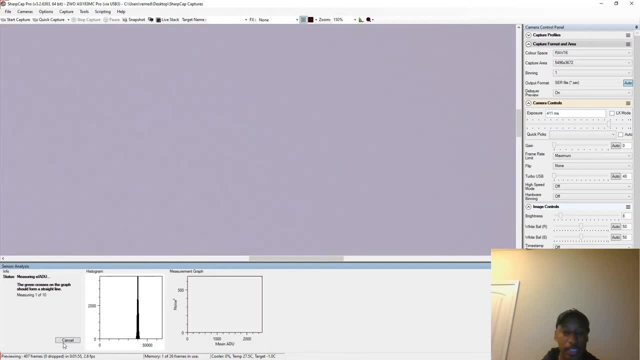 creating graphs doing changes to each of the settings in terms of exposure gain. it's just going to start putting together a chart And from this chart it's going to start creating data for us. This can take some time. it can take. 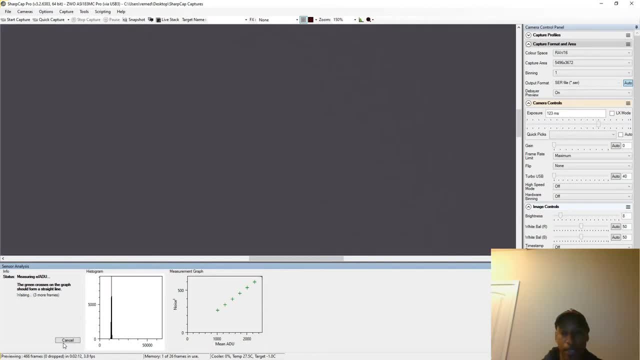 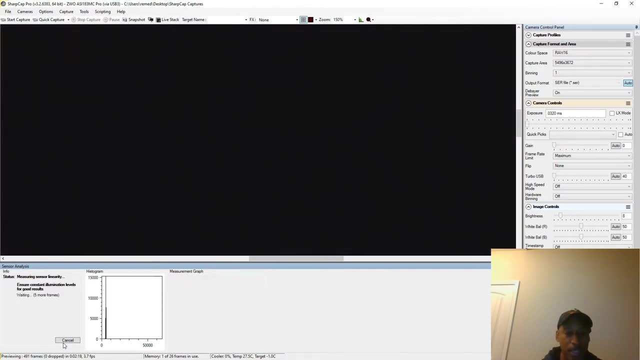 hours. it can take minutes, it just depends on the camera and the sensor. But you know, go ahead and get a coffee or something like that, Let it do its thing And we'll come back. Now it's asking for me to put the cap back on to the sensor, So let's go ahead and do that. 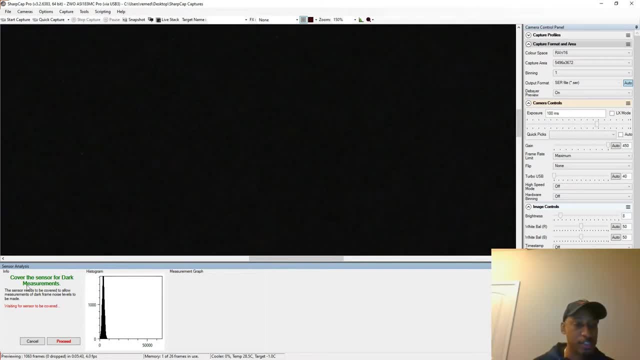 Tap it on, You see again it's changed to green, letting you know that it's ready for you to proceed. And then you click on proceed and it goes through and does a bunch of these measurements Again, now with the cap on. Now it's saying: go ahead, uncover the sensor gain for gain measurement. So again, if 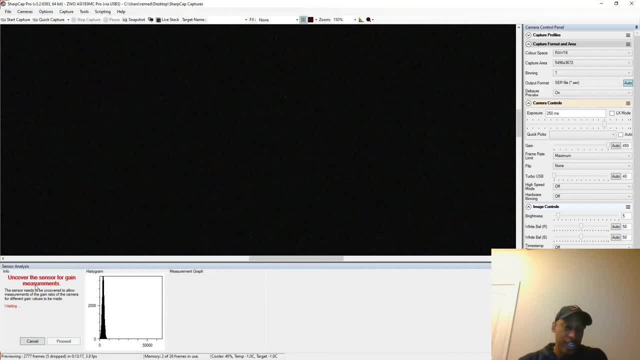 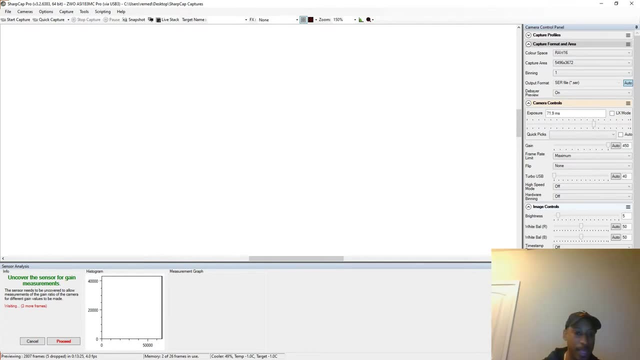 you're looking down here in the bottom, I'm going to uncover my sensor. Nothing else has changed. I still left the five sheets of paper on top of my light source. Okay, because I don't want to change that information or that baseline for this test. 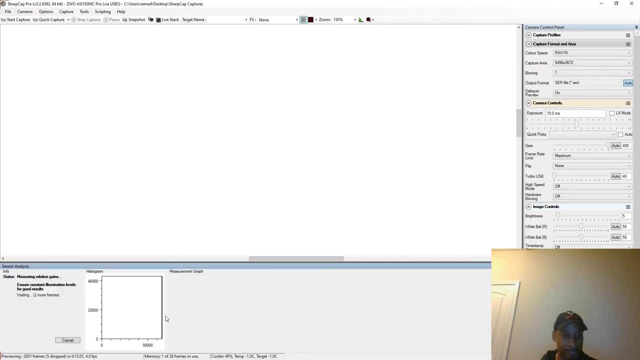 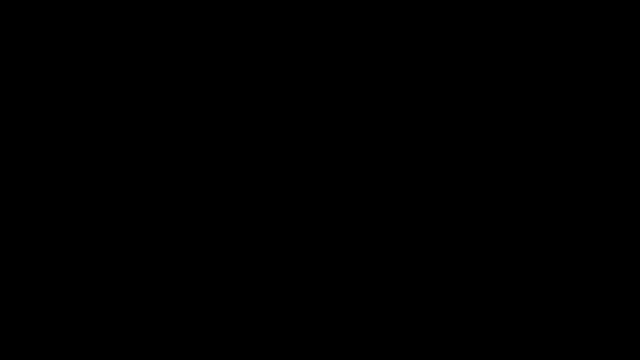 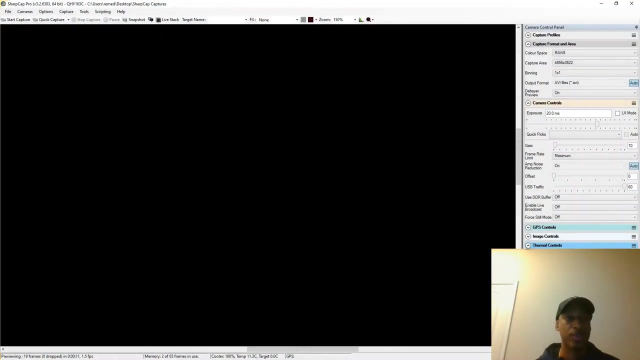 So I'm going to bring it back in and I'm going to hit proceed. Okay, so I've now switched to a QHY163 CCD camera that I have. So between the CMOS camera, the ZWO, and the CCD camera of the QHY, there are some differences. 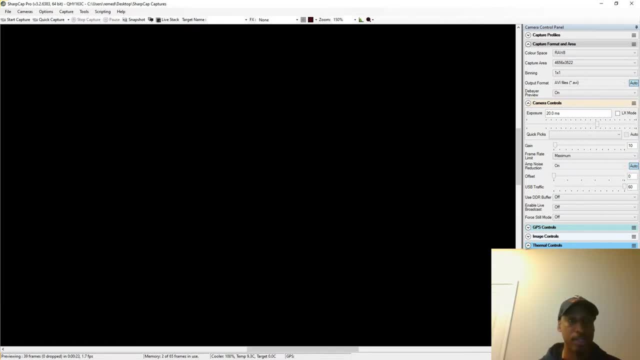 So between the CMOS camera of the ZWO and the CCD camera of the QHY, there are some differences that I want to go over. So before I get back into offset, that's one of the differences you'll see here. If you look at this on the right with SharpCap, it's got an offset bar slider that 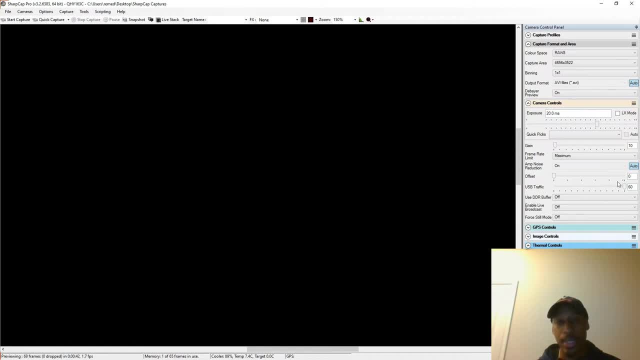 you can adjust. This offset bar or slider is not available with the DCV camera, I'm sorry, the CMOS camera of the ZFUO. So I'm not sure why that is with SharpCap. Some more investigation needed for that. But I wanted to be able to go through that offset discussion with you, So I'm 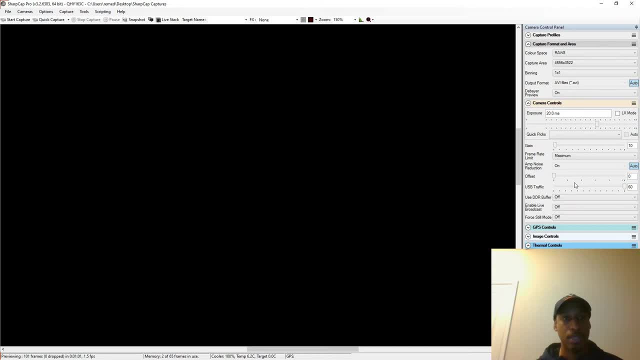 going to take a step back first and talk about a few of the tips and tricks to make sure you get all the way through your sensor analysis. So I had struggles with this particular camera to get all the way through the sensor analysis And what the sensor analysis kept asking me to do was to adjust. 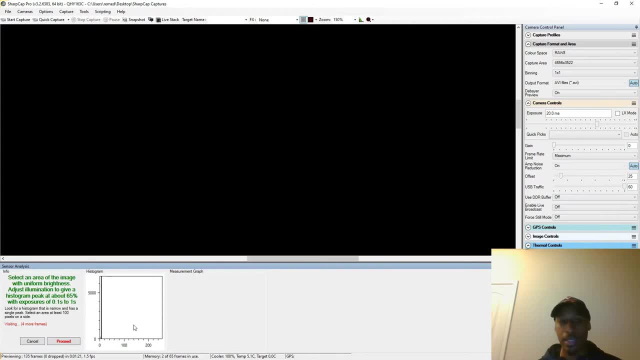 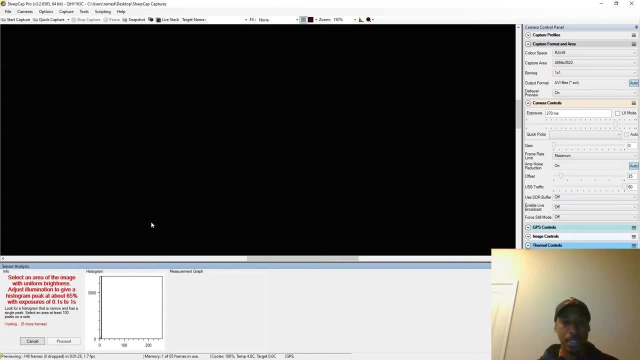 the capture area so that it can measure. do the measurements accordingly. All right, So as I kept making the adjustments that I thought I needed to make, I was not getting anywhere. It kept crashing on me. Okay, So right now I've got the cap on. All right, So cap is off. It's doing its thing, It's got. 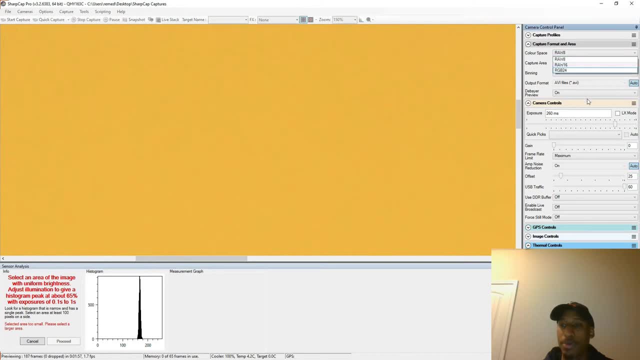 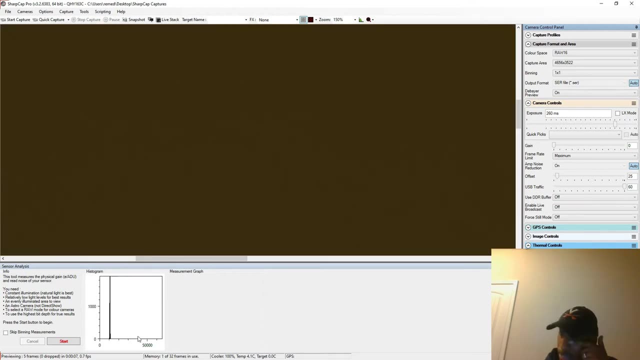 it's not set to the raw 16.. I need the raw 16.. All right, So it's going through the process and it's trying to get it straight, trying to get it straight for this, this analysis. Now it would stop, It would crash, It would get somewhere. It would just tell me: Hey. 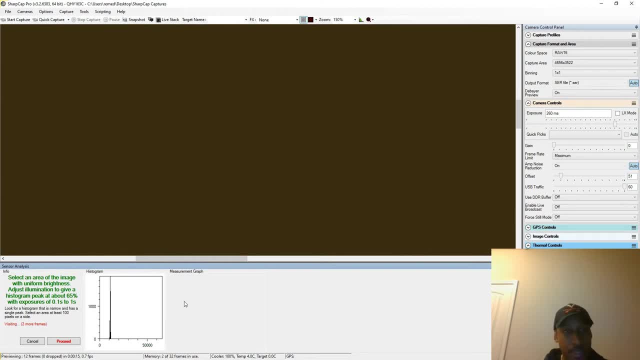 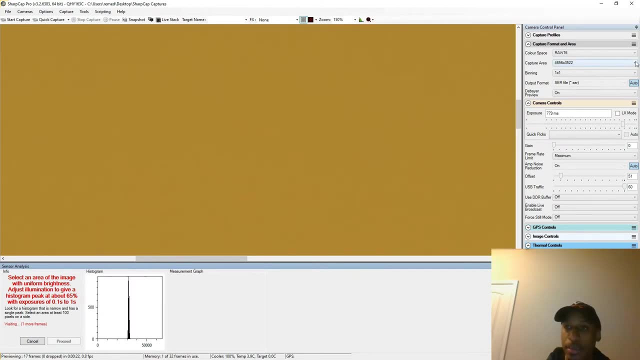 something's not right Need you to change the capture area, and a lot. So it starts off with shrink, shrink, shrink- make it smaller. So if you go over here to the capture area, this is where you can change the size of it, And so what I did in order to get it to go all the way through. 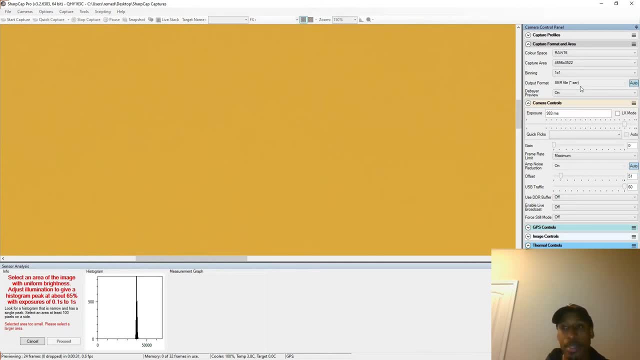 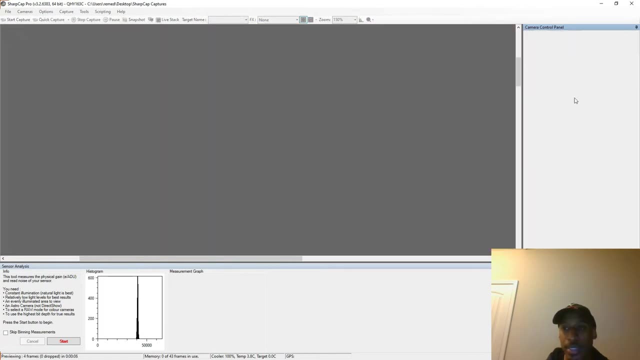 the process without crashing is I would come down one step at a time. All right, I changed the capture area, changed the capture area, changed the capture area. So eventually I think down in this neighborhood. And then, once it got down into that neighborhood, um, it said: oh, 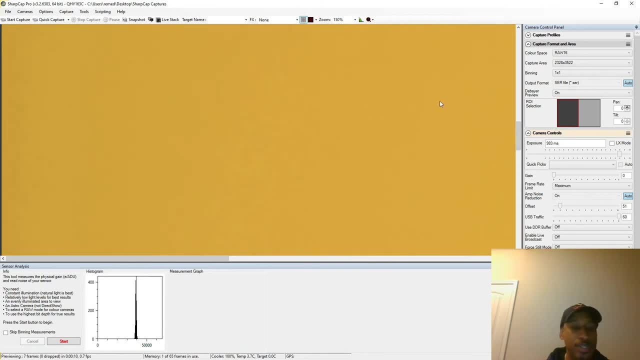 it's too small, I need it to be bigger. Okay, And so, in order to make it bigger, see if this shows up for me. All right, Cause you know intuitively, if I go make this capture area bigger, just going to crash again, Right, I've already seen that, So. so why am I going through? 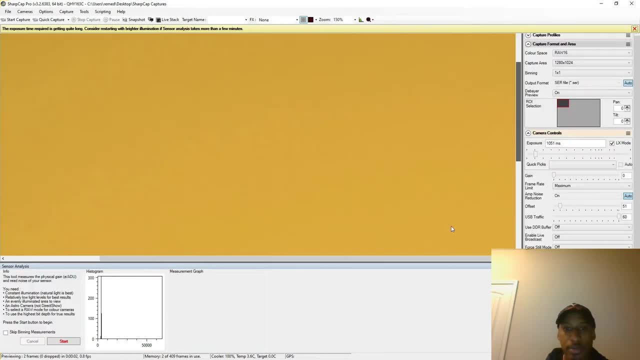 this whole process again of making the thing bigger. All right, Why do I want to do that? So that's not what it's asking you to do. So there is on the screen. there it is this box, All right. And so when it tells you after you've gone through and you shrunk it. 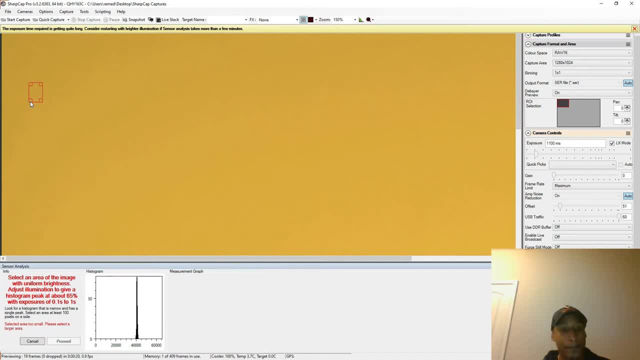 you shrunk it and shrunk it, and then it comes back and it says: okay, I need you to make it bigger. What does that ask you to do is to go in and change this capture area here now to something a little bit bigger, And so you do that until this goes green. 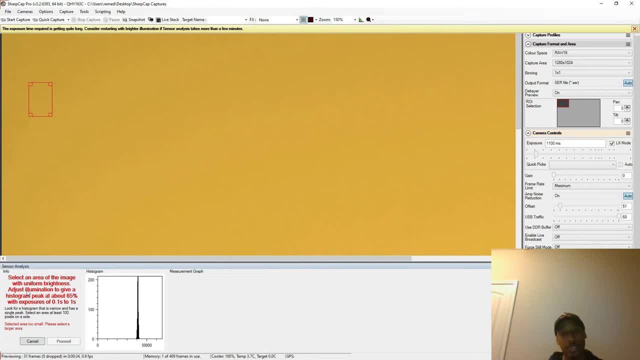 boom, and then you're done. Now you've dialed it in and it will go through the entire process of camera. So if you got like me, if you had that issue where the QHY 163 would not go through the entire sensor analysis, it would keep crashing, It would keep airing out. That's what's happening. 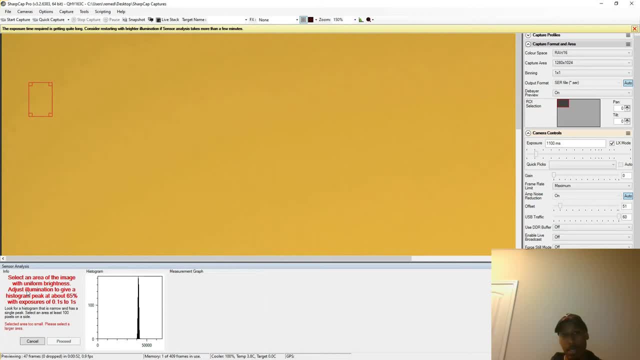 is. it's asking for you to get to the right size um surface area that it's looking at, that has even illumination all the way around it And, um, and even what it says here, it's got a hundred pixels on each side, right? That's what it's asking you to do. Um, that's a. 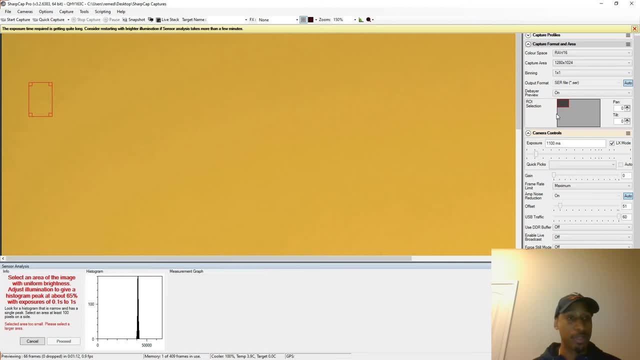 little difficult to just predict what it's going to be off the bat. For me, it was a little bit of a struggle trying to get to that point, And so that's why I'm suggesting, if you run into those same issues with your camera, you just want to keep changing the capture area down one by one. 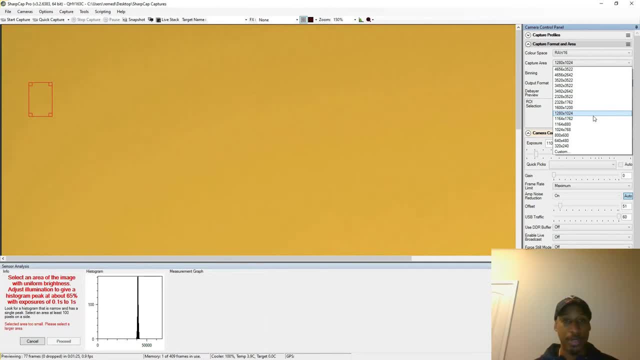 by one until you get to the point where it then says: oh, I need you to make it bigger, And of course you don't want to make it bigger here, You want to make it bigger in one of these boxes. You could even move this box anywhere you want. Okay, On the on the screen. All right, And once you've 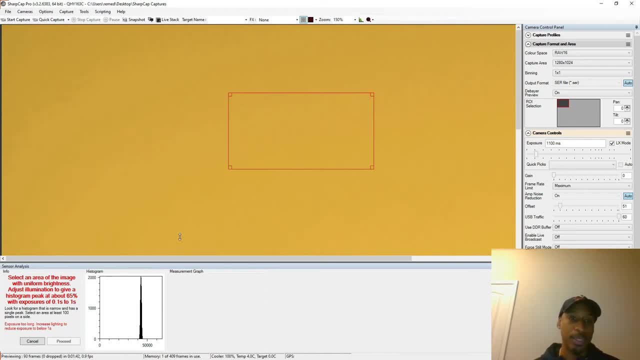 go green, then it should be able to go all the way through the process: complete your analysis, capture your data, put it in your Excel spreadsheet and do things you need to do with it. Okay, All right, Good, So, that being said, um, let's talk about offset. So I'm going to put 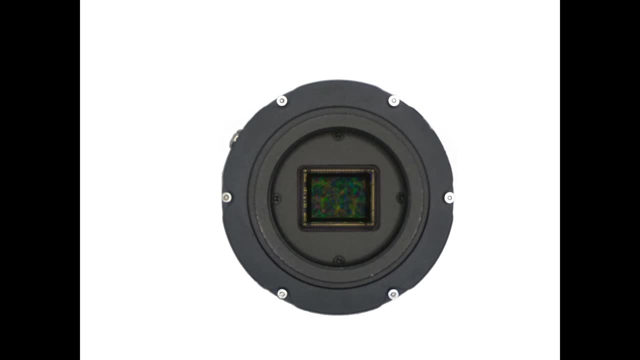 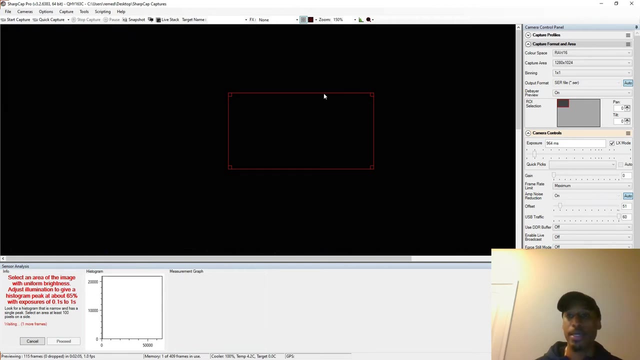 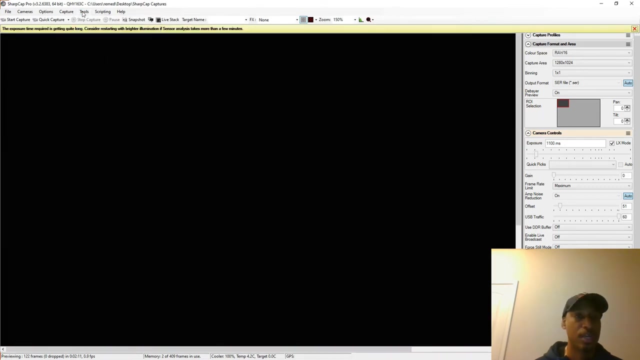 the cap back onto the camera, And I think you can do this with more than the shop sharp cap. So if you're the ZWO camera, um has the offset capability. uh, that you can deal with in other tools, um like, uh, Ashton photography tool, which I haven't done. 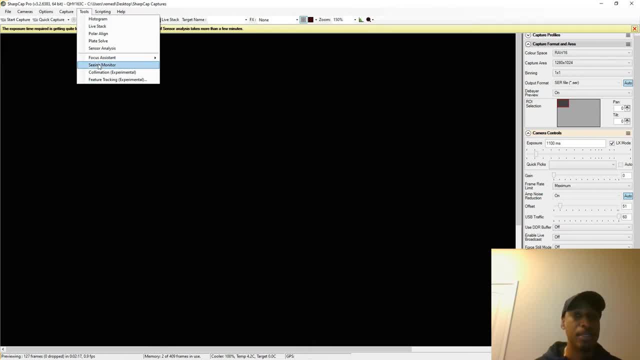 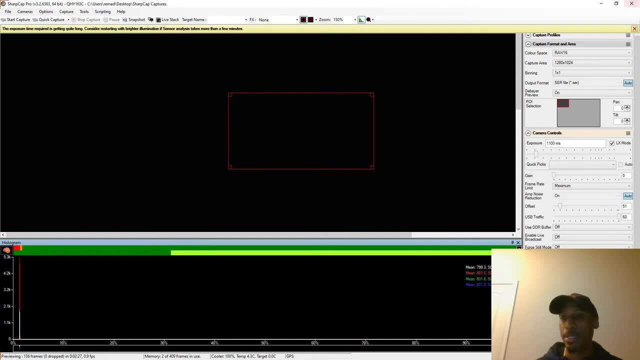 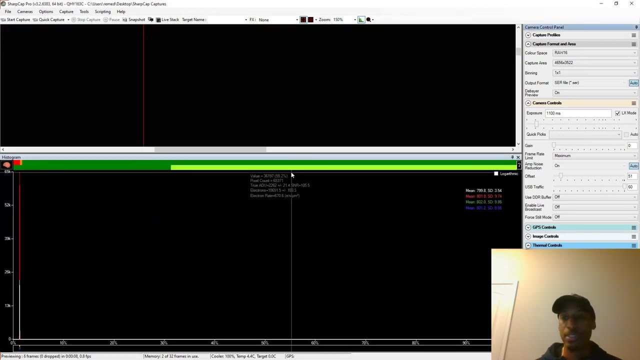 So I'll try that here later. Um then, you can go through this process, but since I've got this, now I'm going to go through the process with this camera and I'm just going to make the capture area as big as possible again. And so what the histogram is showing you are three different. uh, three. 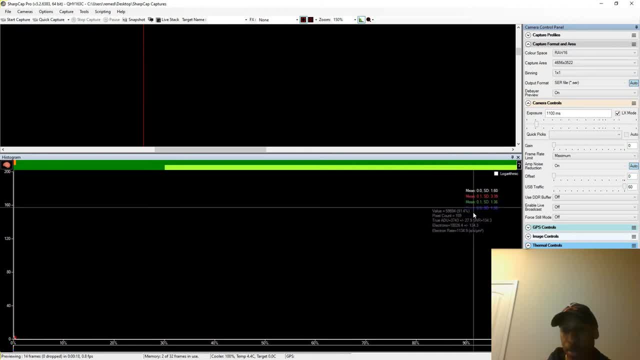 different histograms. So before actually you've got the mean of all three of your colors: red, green and blue. Okay, Looking at the mean, that's going to be the white bar, the white histogram on on the left here. 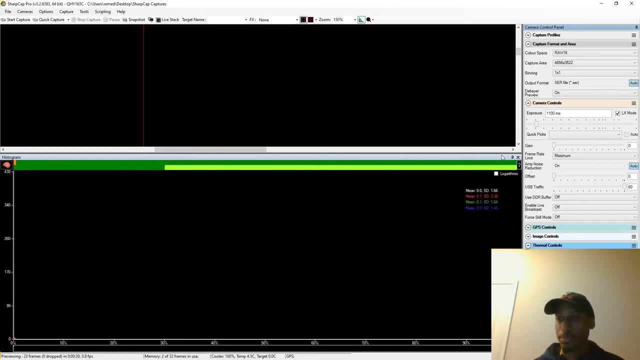 Okay, And so at zero gain. if my gain is zero, right, I want that histogram to sort of come off of the end. Okay, So let's try. let's try 10, and you can see over here to the right. it came off. 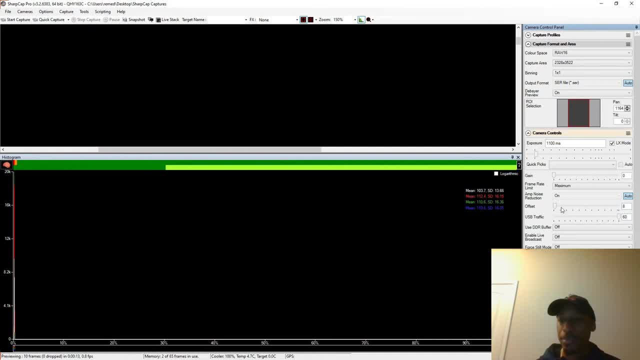 of the edge, um, appropriately, And so from a offset standpoint eight, move the histogram over. So the mean histogram is over. It's completely showing uh, no tails or anything like that, cut off by uh on the left right. So 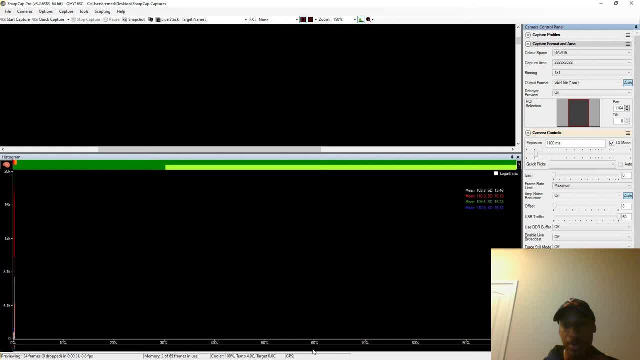 that's clipping, So you don't want any clipping. You got all of your data right where you want it to be, uh, in that histogram, So let's just change the game. So again, uh, if you go back to 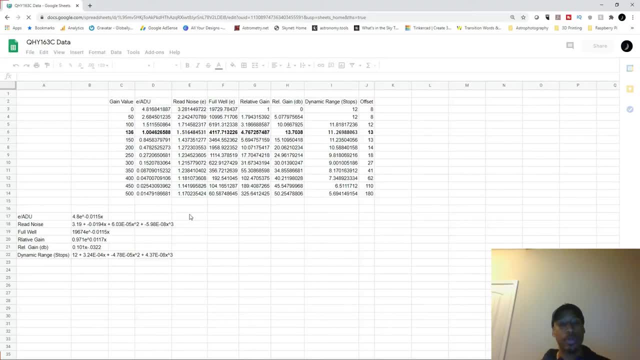 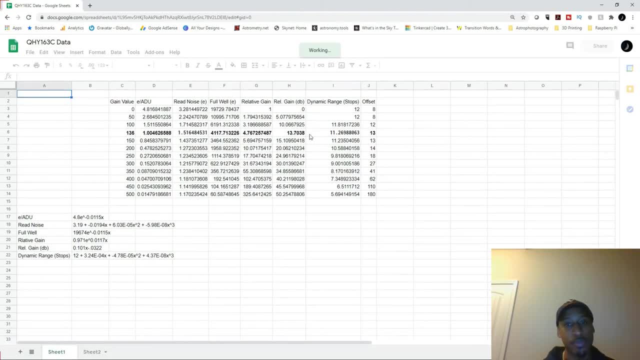 I've just gone through the process, at each of these different game values and look to see where my histogram- the average- was not being clipped. Okay, So long as the average is not being clipped, that was the minimum offset- not maximum, but minimum offset that I would choose for each of. 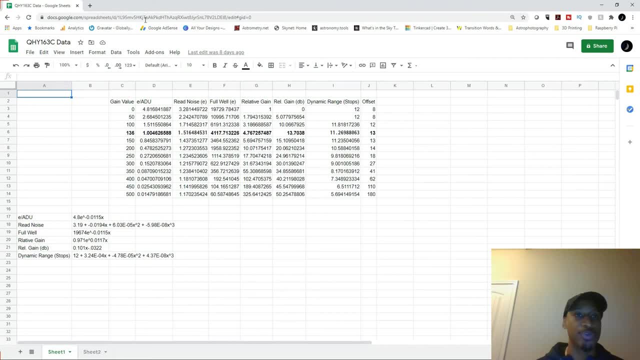 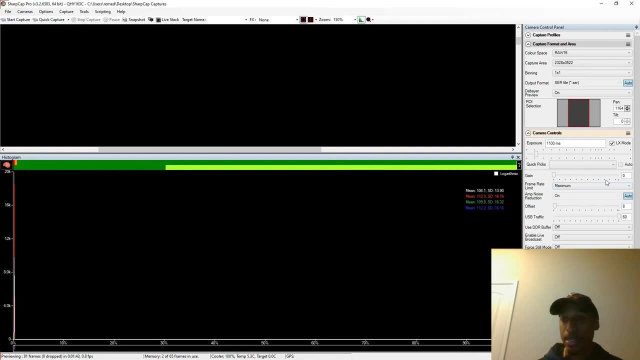 these different game values, Okay. So let's go back to tarp app. Okay, And let's choose a higher gain. So I'm going to choose a gain. I'm sorry, And I get, yeah, higher gain gain. all right, now i've got a higher gain, i want to move that as well. so, again, it's very hard to. 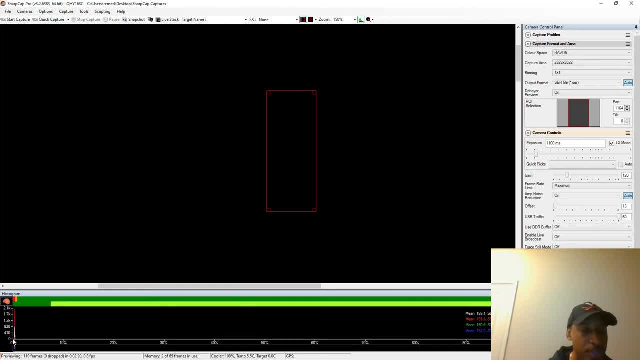 see on this particular graph. um, but you want to make sure that that average is as far over as possible. okay, not clipping on the left, and you can. you can look at your numbers here as well and try to see whatever method you want to use to determine whether that's true for you. um, that's. 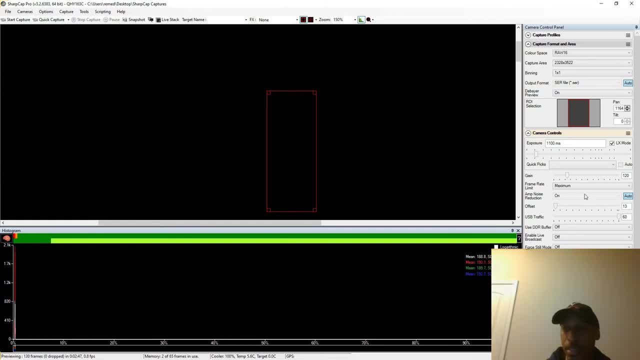 what you would do. so, um, yeah, so as, and, and all, that's all i've done for each one of these. i've just changed the offset. i changed the gain, change the offset. when i change the offset, i'm looking for that average histogram to not be clipped on the left here. all right, and so i did that, for i'll. 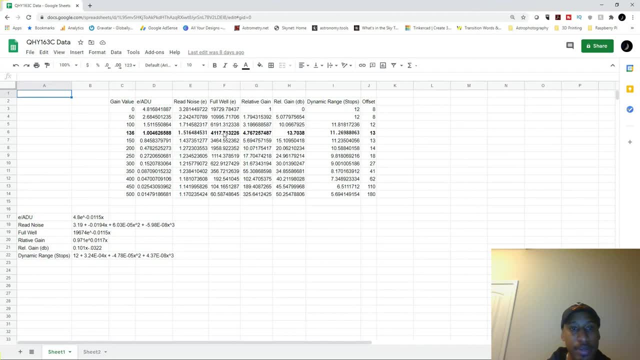 close this right now. so i did that for every gain value i have here, which includes my unity gain, which i didn't know was 136 at the time, um, to show it as 13. so i've got my offsets all labeled out now. the higher the gain is, the more forgiving the offset numbers are. so 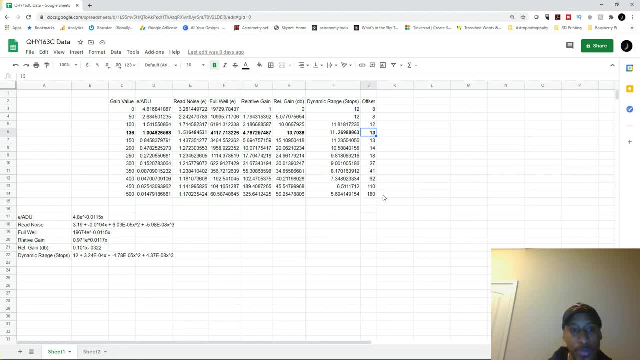 there's a larger range of offsets you can choose from uh for, let's say, the 350 gain value. if you wanted to do a 350 gain, i'm doing 41, but as i kept on changing the offset number the instant, the histogram uh didn't change a lot. so there's a lot of range between a 40. 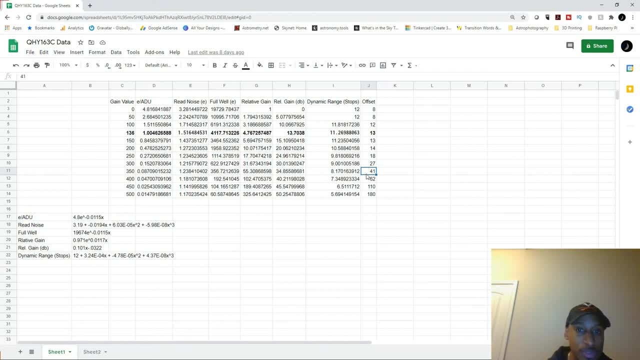 and probably 70 that i could use as offset. so it becomes less of a factor the higher the gain. you don't need a whole lot of offset to deal with. not that i i'm going to be going at such a dim targets that i require 500 gain value, but just as a piece of information for you you can actually go. 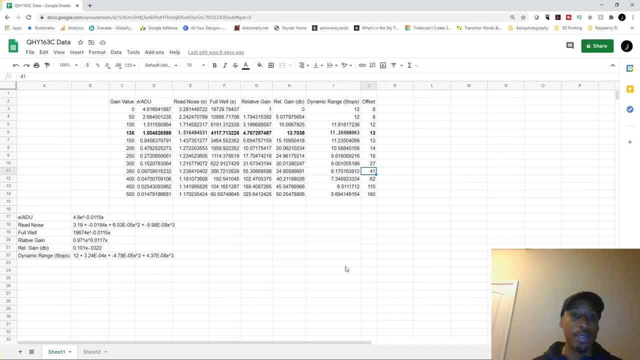 through and set these offsets using the histogram and just making sure that you're not clipping any data. whatever that minimum number is is what you can start with. you can always go higher. you can move the insta histogram anywhere you want. i keep trying to say instagram. okay, so that's offset. 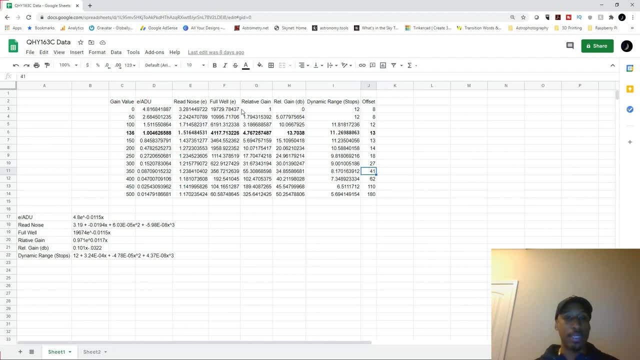 already has to start trying to look at capture offset. like i said, i will work on a video for explaining gain and offset and how to use them with your camera, because that's important. in the meantime, of course, there's a lot of uh optional um videos on youtube that show you an. 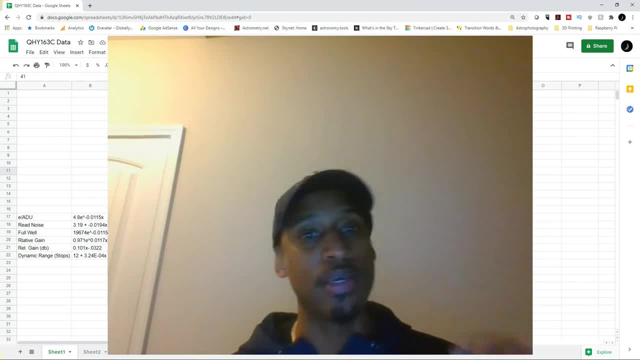 example of how to do the same thing, um, but, like i said, it's a lot of great stuff, so i just wanted to to give you some other tips for joining the team. if you're still with us, keep playing the game and keep watching. hopefully this helps you, and remember: the sky is always the limit when your